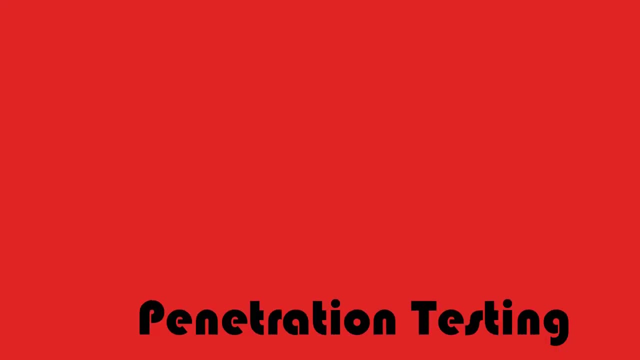 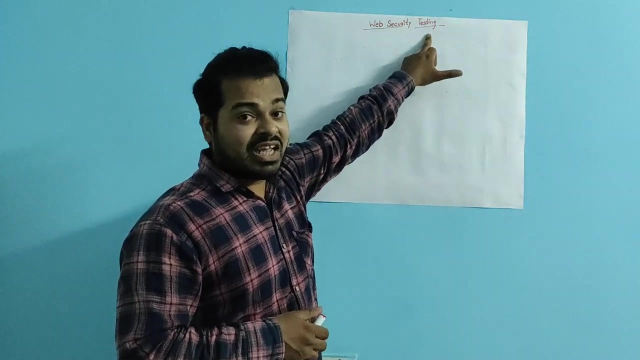 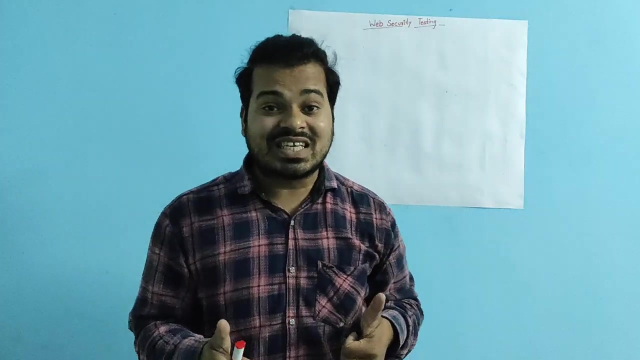 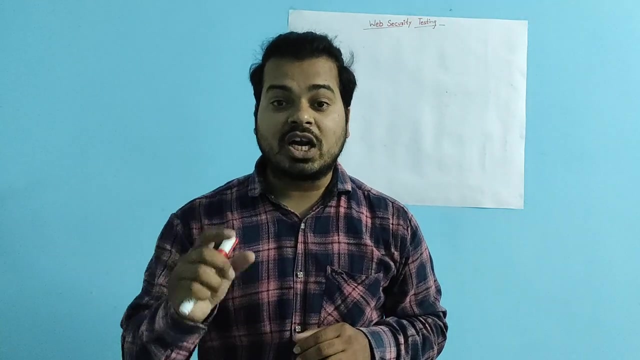 Web security testing. the other names are penetration testing or fuzzy testing. So, as the name suggests, it is a type of testing we do in the web application to test its security, how secure it is. Definition says that testing the authentication of an application to test how well the application is secured from the unauthorized users or hackers is called as web security testing. 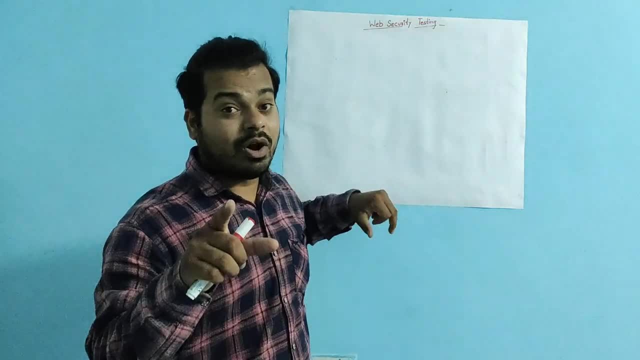 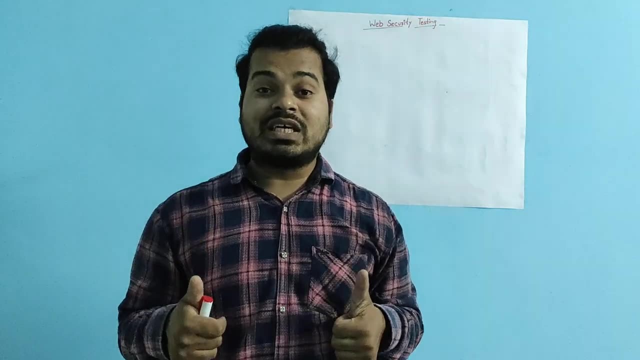 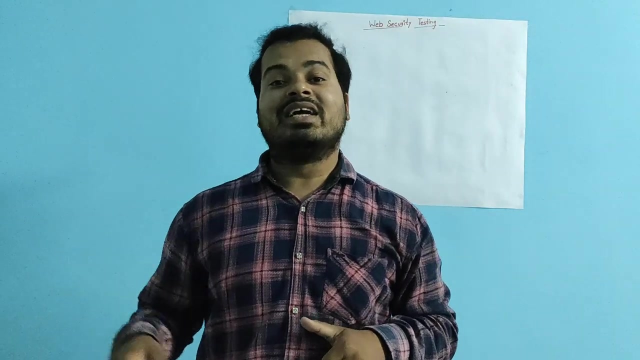 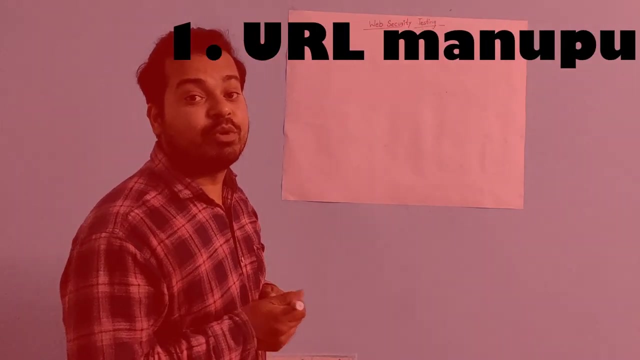 Testing, also called as penetration testing, also called as fuzzy testing. These are the other names, Guys. at the end of the video I'm going to tell you guys what are the questions in interview they can ask regarding this topic. So make sure that you watch this video till the end. Let's get started. The first type of web security testing is called as URL manipulation. 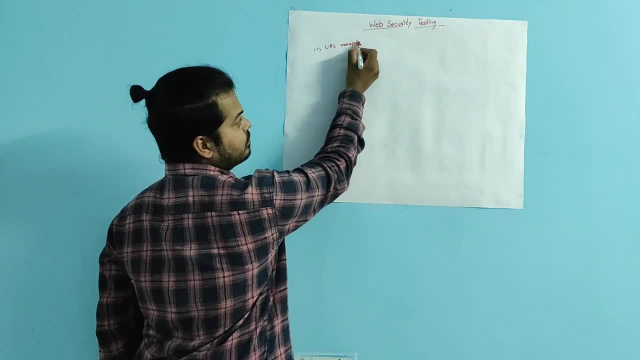 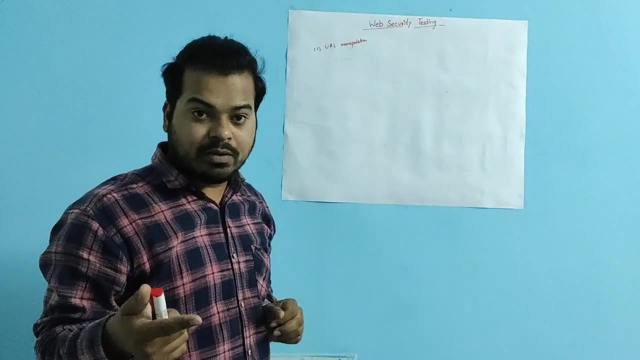 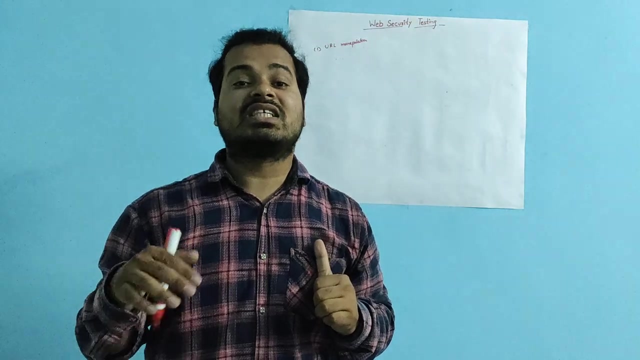 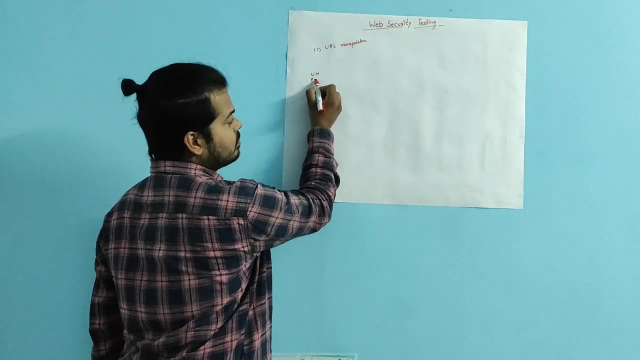 So URL manipulation is a type of web security testing in which user will log into some web application using his credential, Let's say username or password. He has entered his username, password and he has logged in After going to the login page. suppose this is. I'm talking about a web security testing? 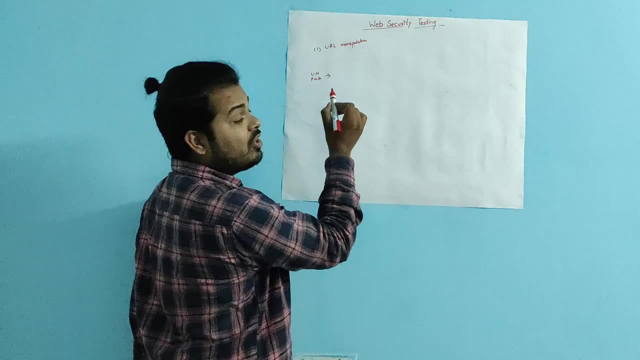 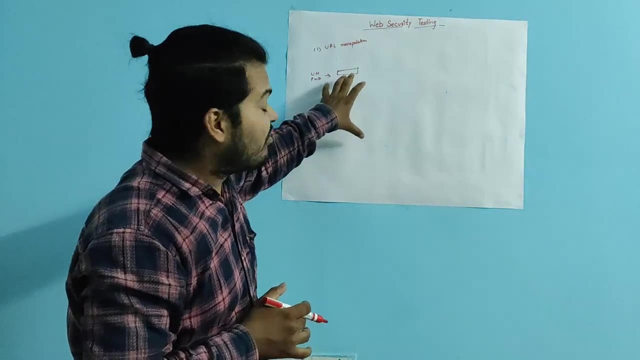 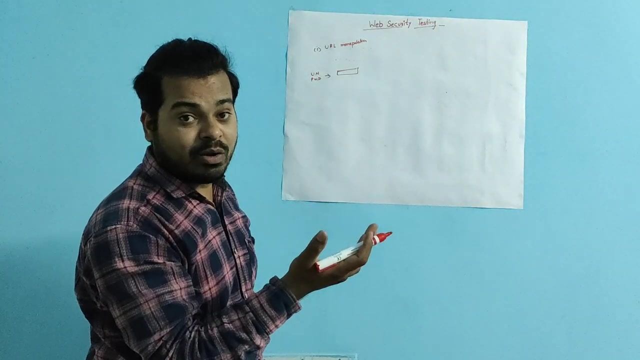 Then he has clicked on compose a email. He has clicked on it and he has typed a mail. After that, what he will do? He will copy the URL. If you are trying to access any browser, definitely a URL will be there, Right, guys? 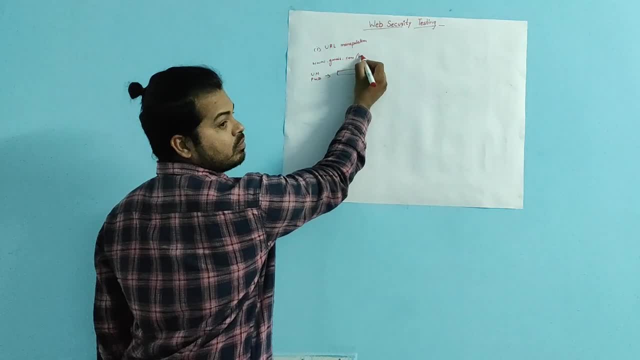 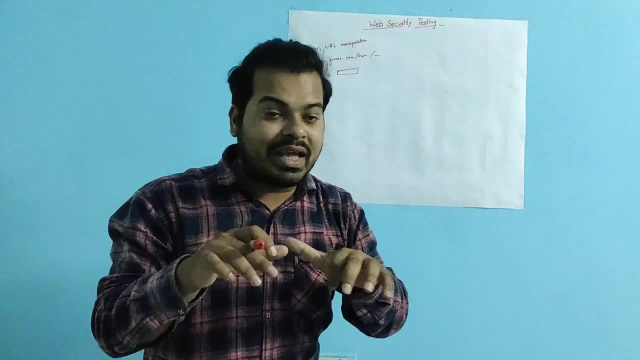 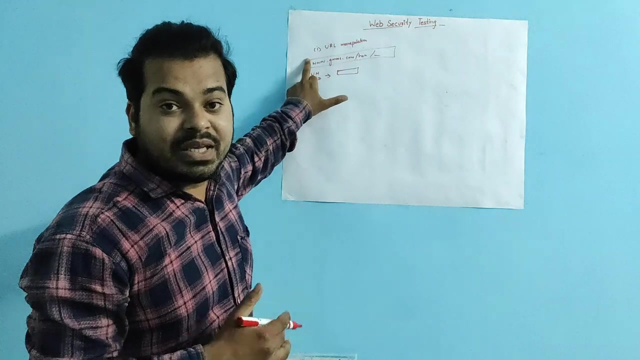 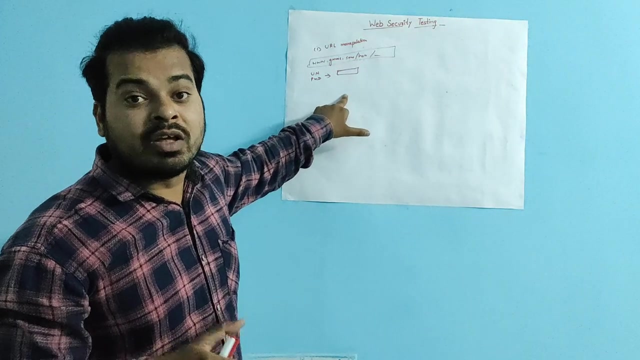 wwwgmailcom. slash home, slash something, slash something. something will be there, right. so, after clicking on compose button and writing his mail, he will copy the URL and he will paste it in his notepad. again what he will do: he will log out from the Gmail application. once he has logged out, 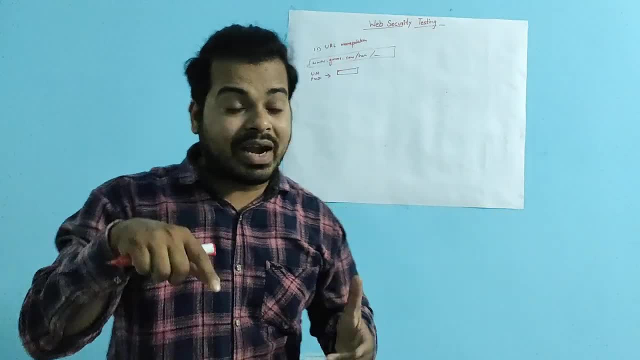 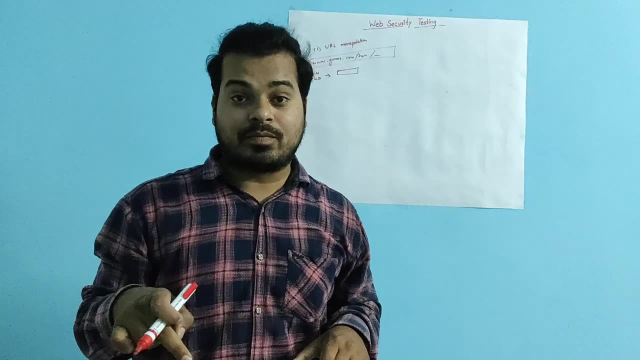 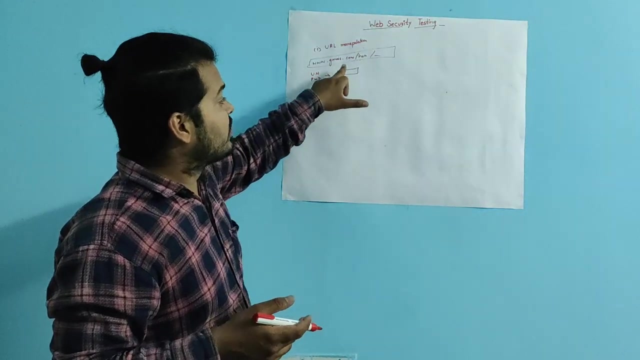 he will copy whatever was there in the notepad- the same URL- and he will go to the browser and paste it there and and he will click on enter. if my new URL is allowing me to go to the same compose page, that means it is a security defect. 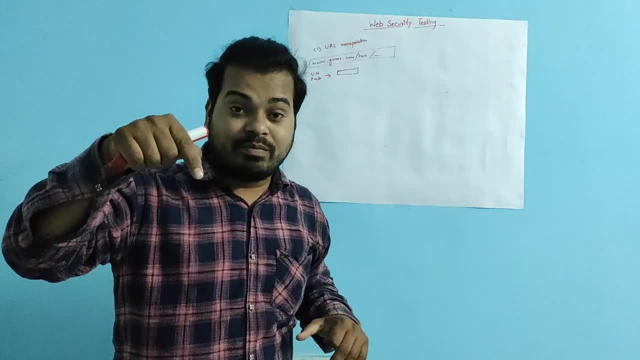 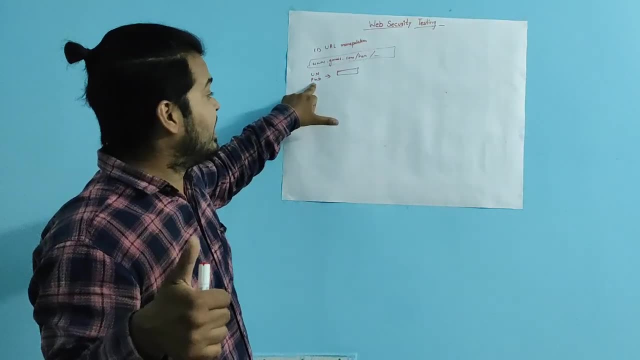 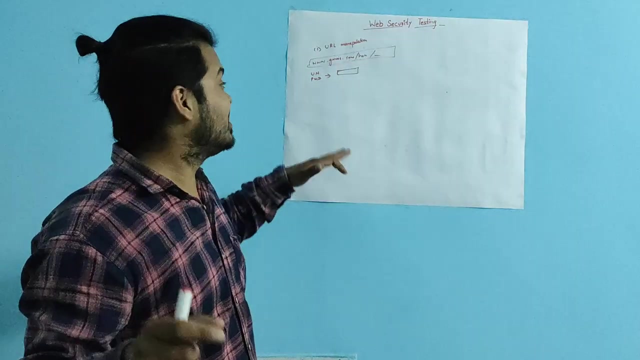 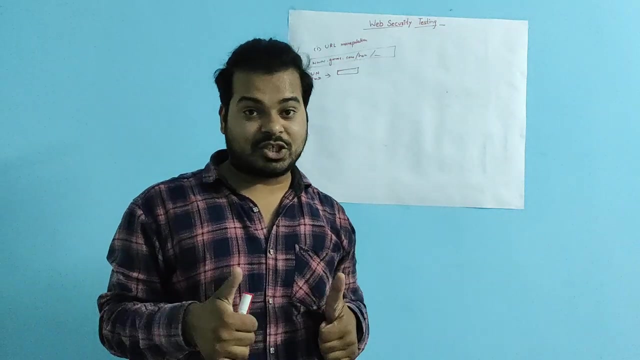 but while launching that URL, if my I am redirecting to the login page where it is asking me to enter user name and password, then we can see the URL is there, say that it is highly secure application. this is the first type of web security testing called as URL manipulation. I hope you guys have understood. let's get. 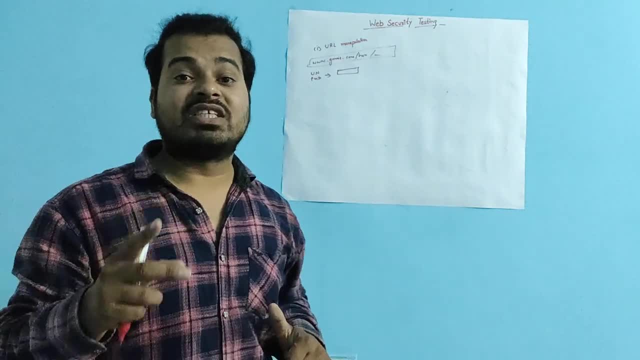 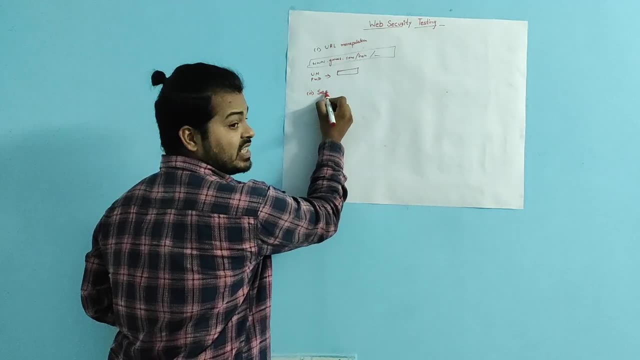 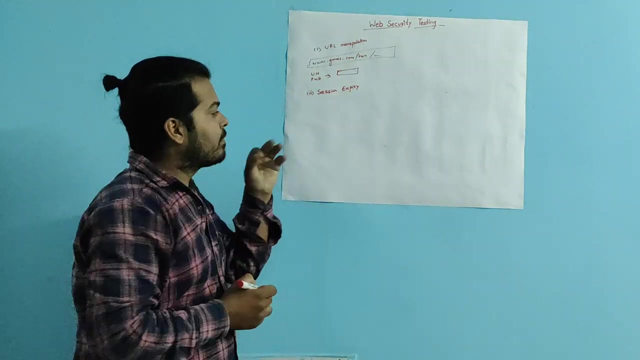 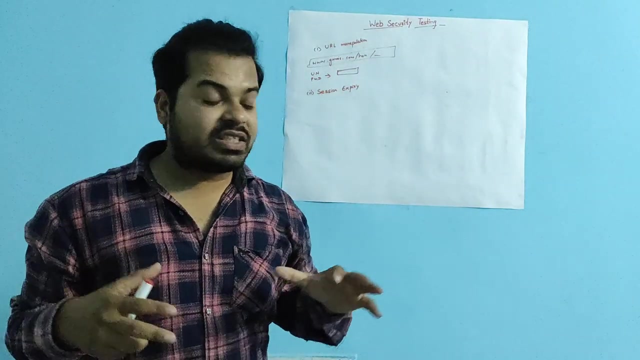 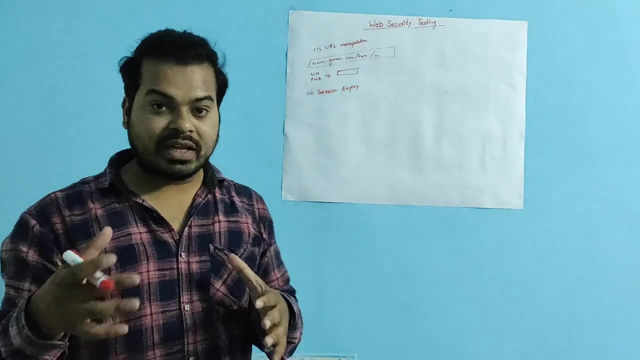 started with the second type of web security testing, which is called as session expiry. session expiry. session expiry is a type of web security testing in which- so this testing usually will be done in some bank applications, so where you are logged in in the application and you have, you have not. after log logging in, you have not. 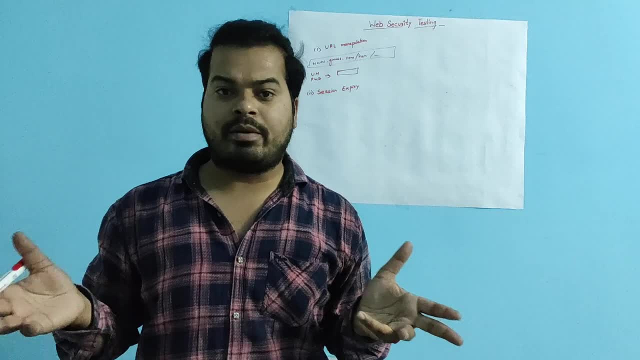 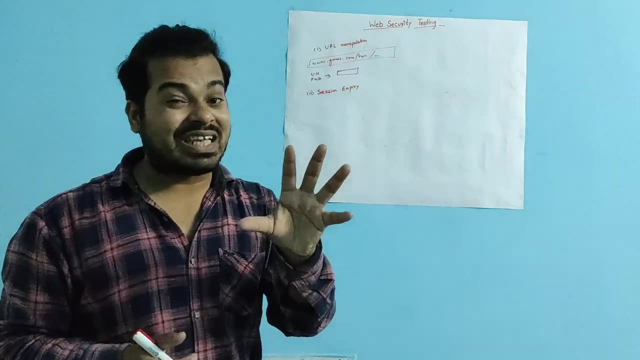 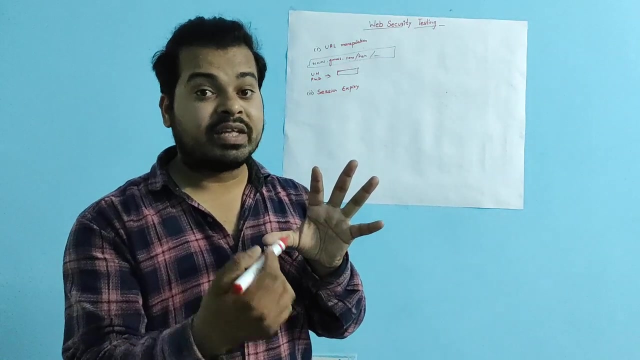 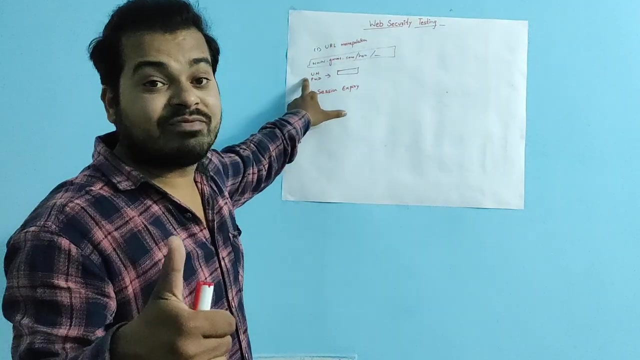 done anything you. you have kept the application idle for more than five minutes, let's say. then it should display pop-up message saying that you have done well. session has expired with a button called as okay. if you click on ok button, it should take us to the login page again. if it is taking to the login page again, it is. we can say that. 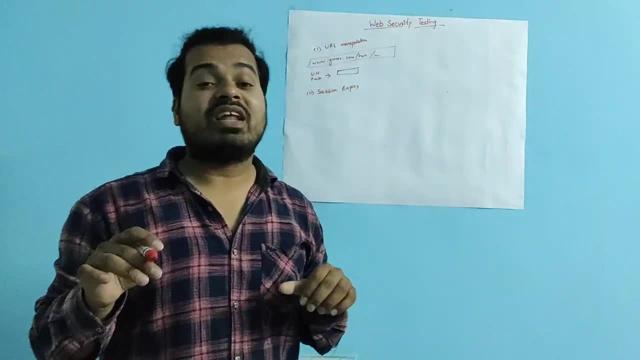 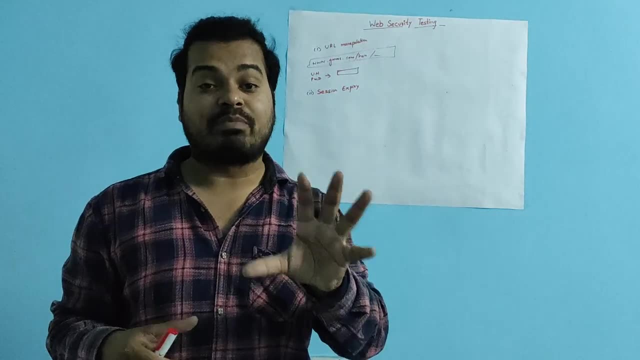 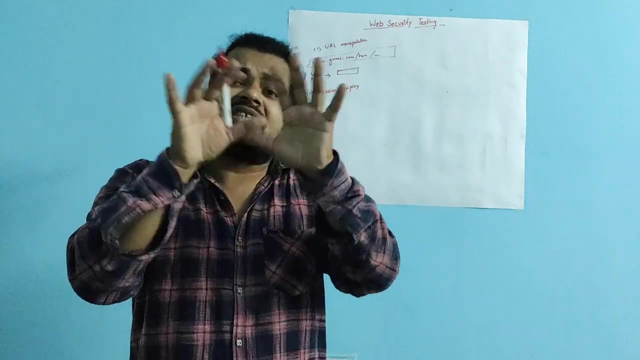 it is a secure application. but even after leaving the application idle for more than five minutes and pop up has come saying that session is expired, with a button called as okay. but if you are clicking on ok it is redirecting to the same page. it is on the same page. it. 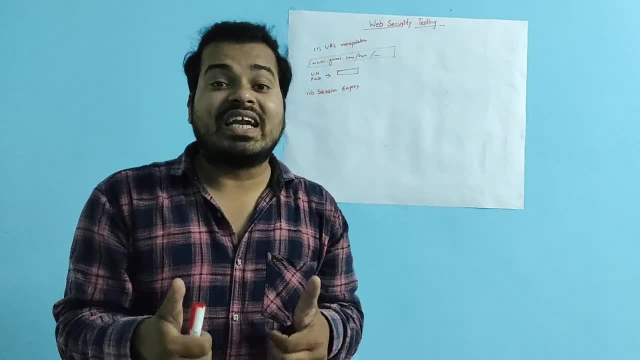 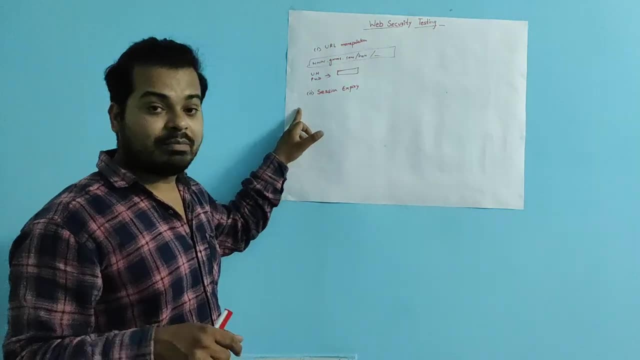 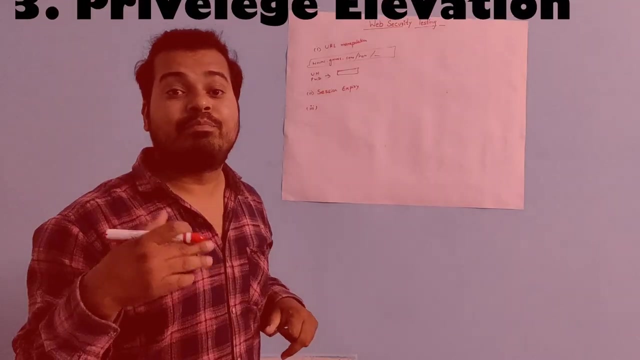 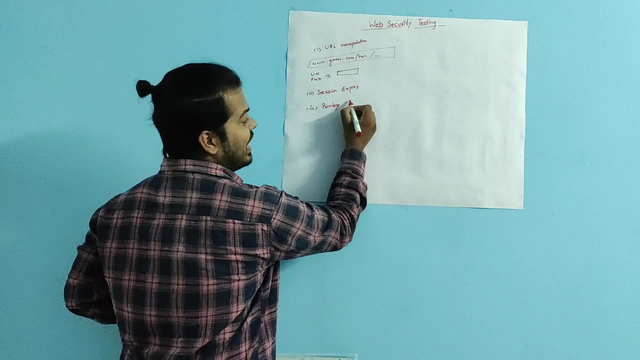 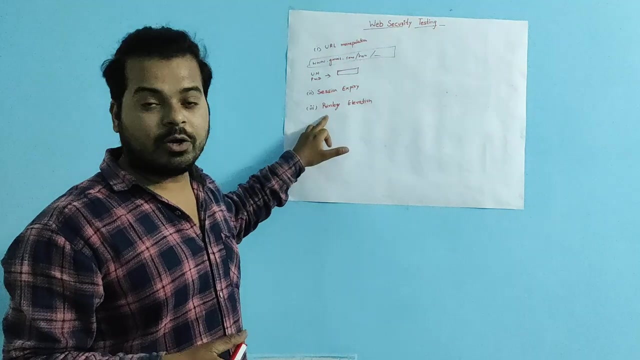 is not redirecting anywhere else, we will say that it is a security defect. we will say that it is a security defect. i hope you guys have understood. coming to the next one, the third type of web security testing is called as privilege elevation, privilege, privilege, privilege. so, guys, what do you mean by privilege elevation? suppose i am a hacker who is having a account. 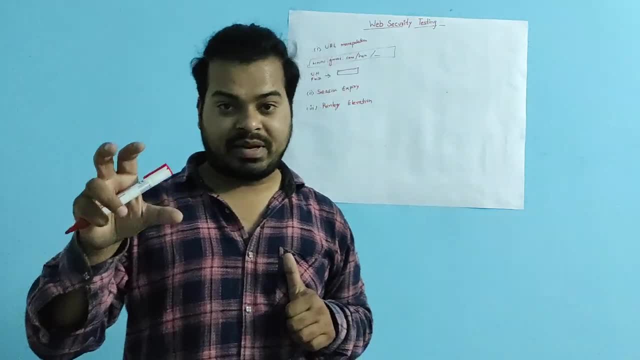 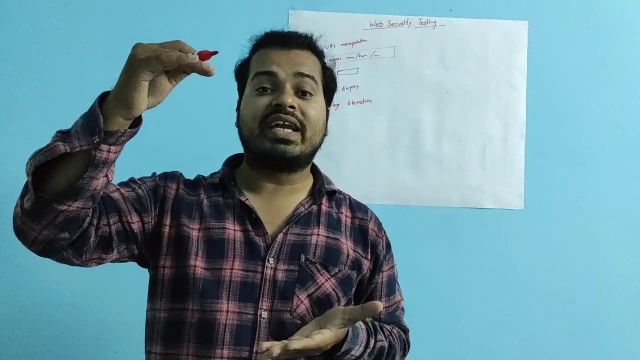 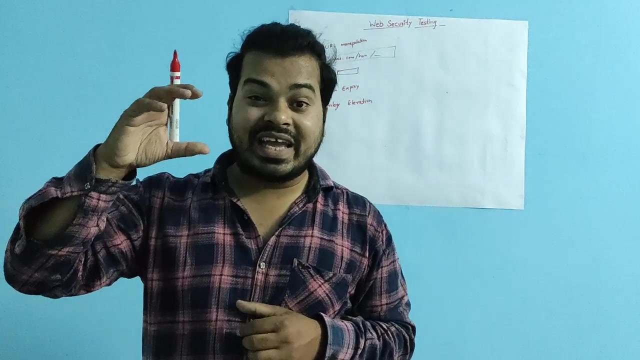 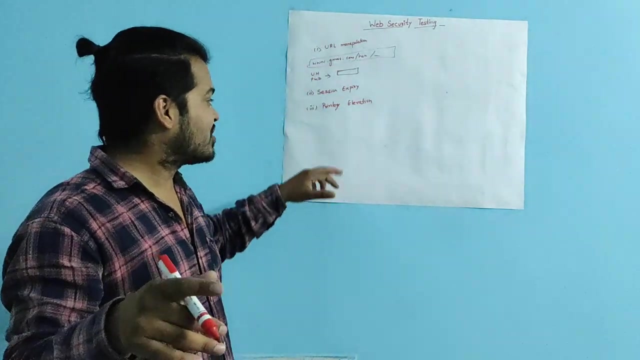 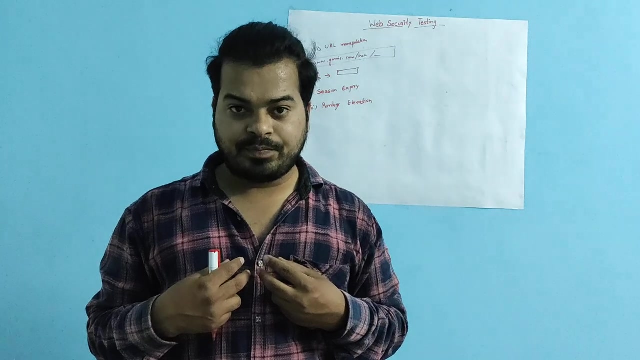 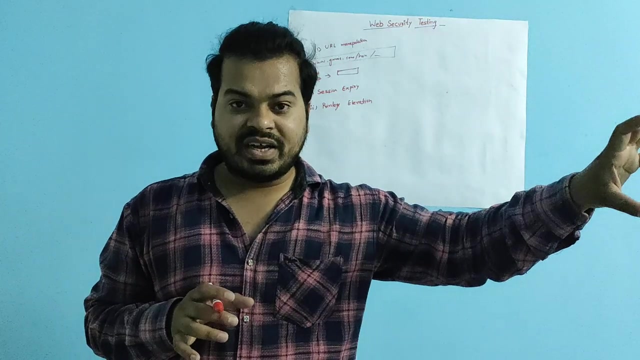 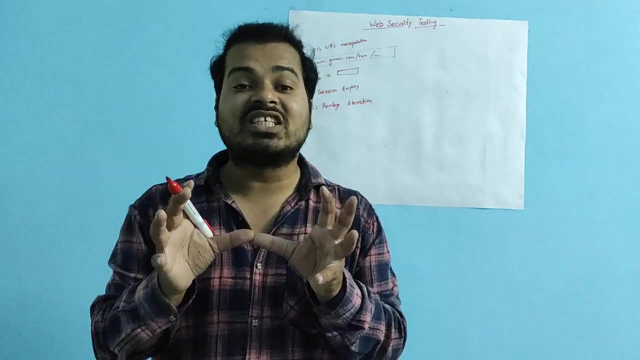 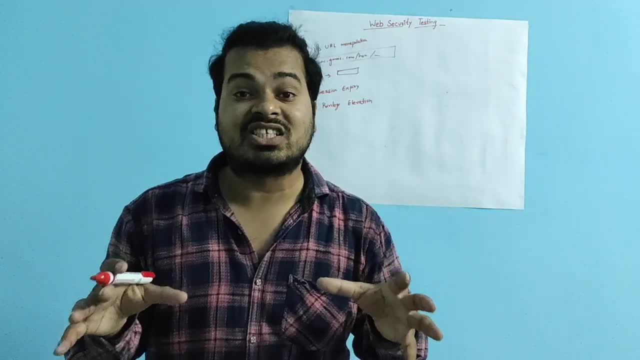 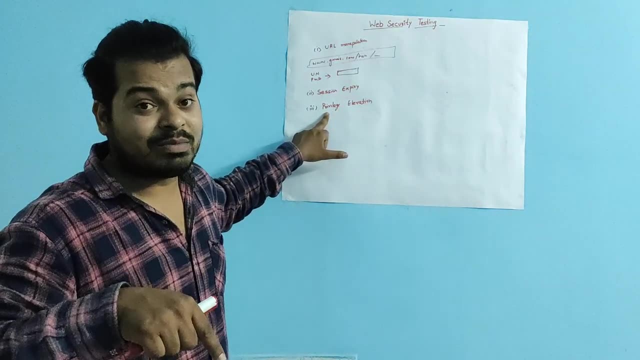 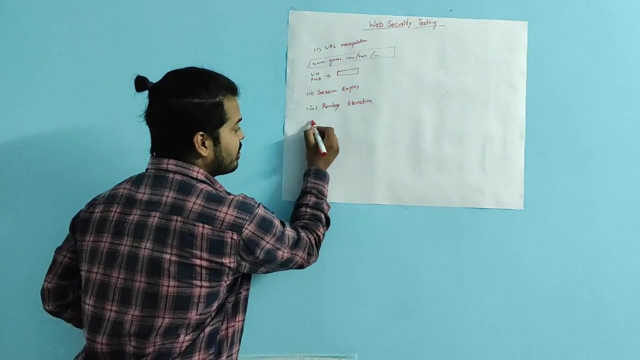 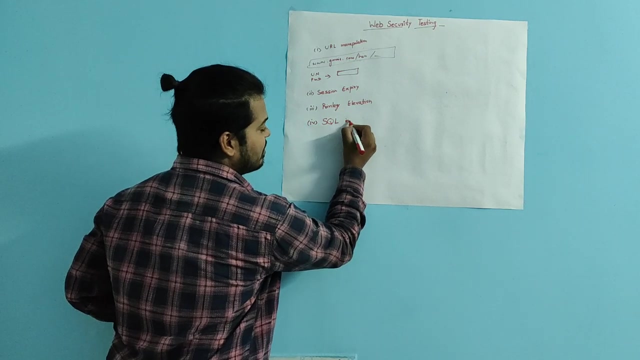 call the resident manager then i need not ask his permission for each and everthing. stop stuff i do. that is called as privilege elevation. i hope you guys are. if not, list out in the comment section i will answer. let's go to the fourth type of web securely testing. it is called sql injection. sql injection is a type of web securely testing. 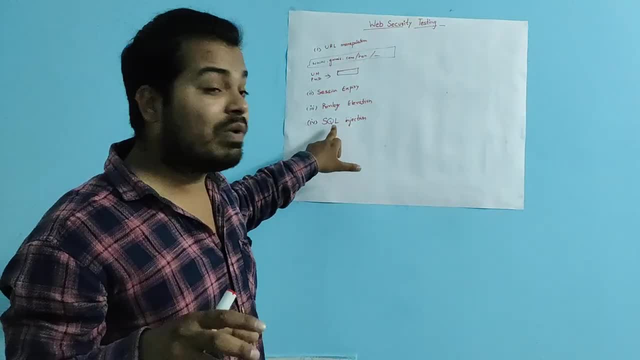 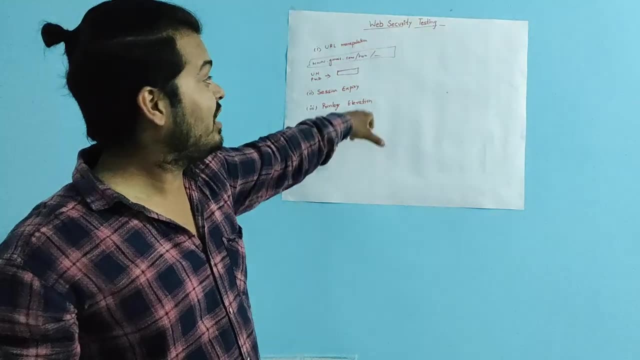 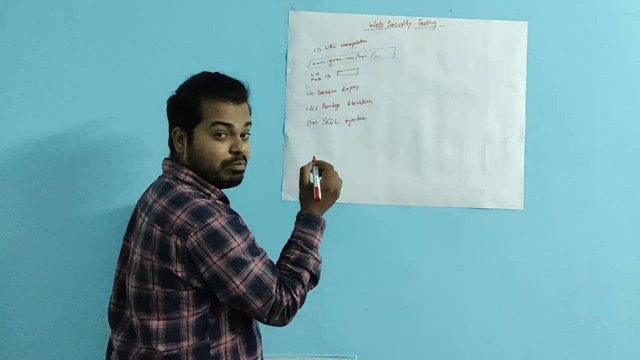 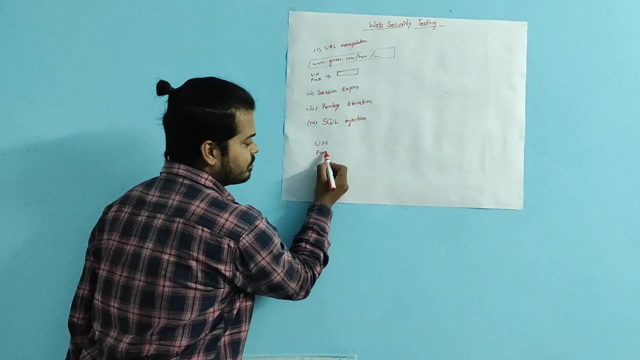 testing in which hackers will inject SQL commands into SQL statement. that is called as SQL injection in web security testing. now the question arises how let's get started. suppose I am having an application in which I have to login with my username and password whenever any user in this world he is using any 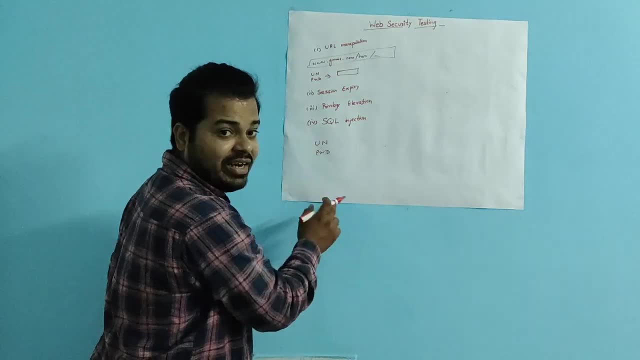 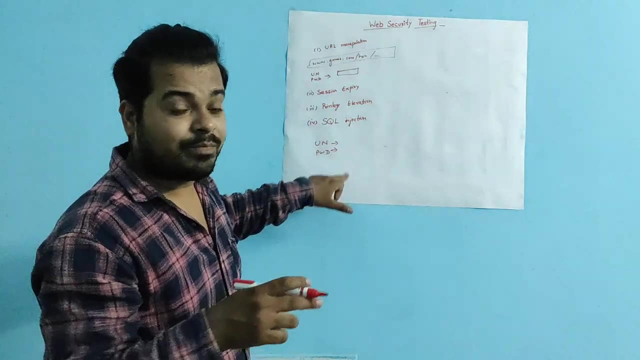 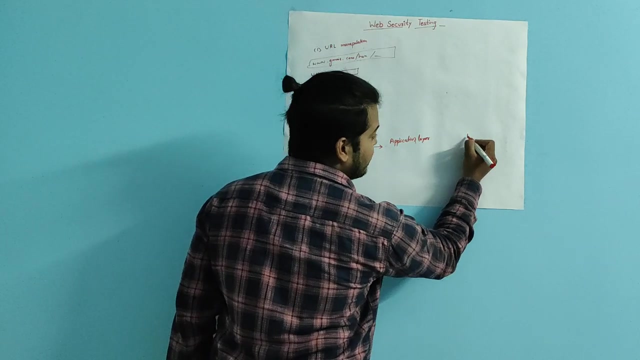 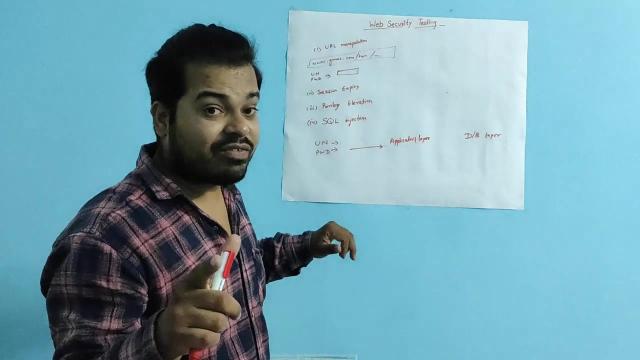 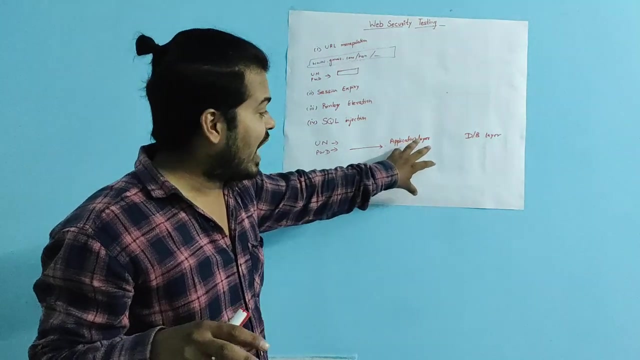 application. he is having a UI right where he will enter his username and password. once user has entered his password, it will go to the application layer, database layer. whenever user will enter username and password, process will happen in application layer and it will try to get the information from the DB. that is. 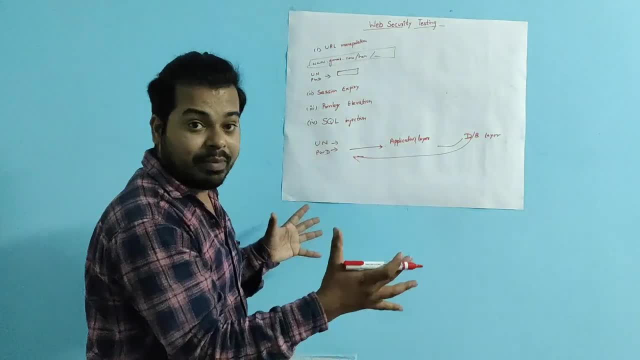 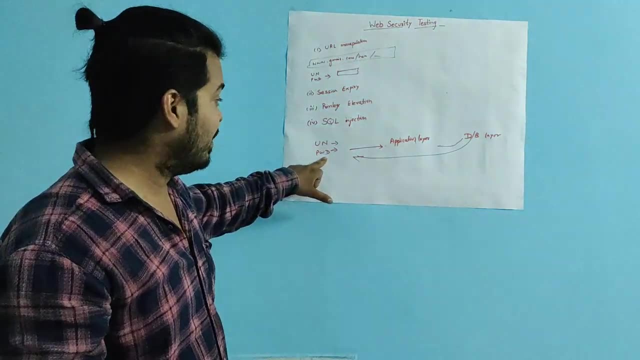 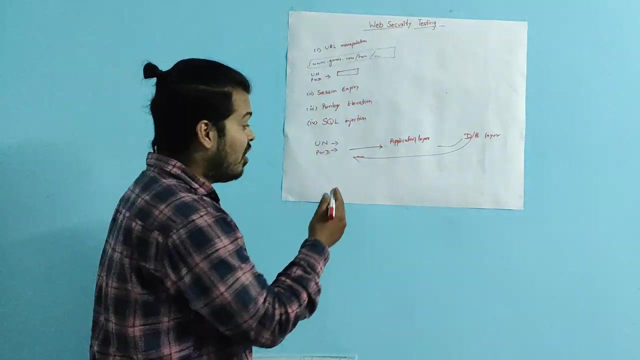 database and then account will be opened. this is how normal users will do. will open his application. but in sql injection, what user is going to do? what hacker is going to do? hacker will not enter his password correctly. he will write some SQL commands. he will write some sql commands and the user will be called as a hacker and he will be called as a hacker. 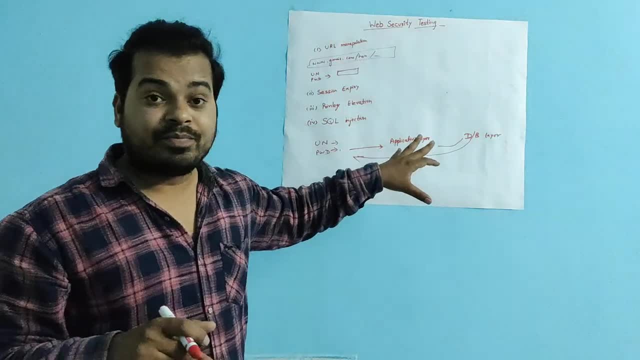 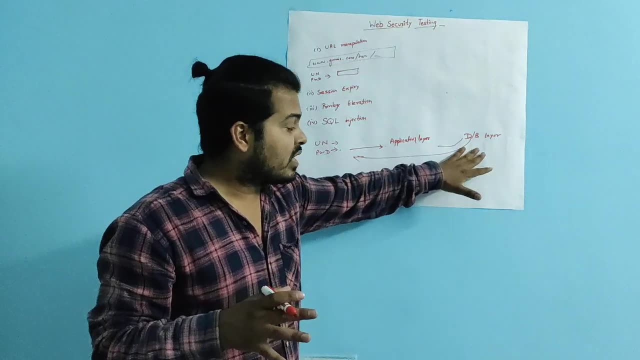 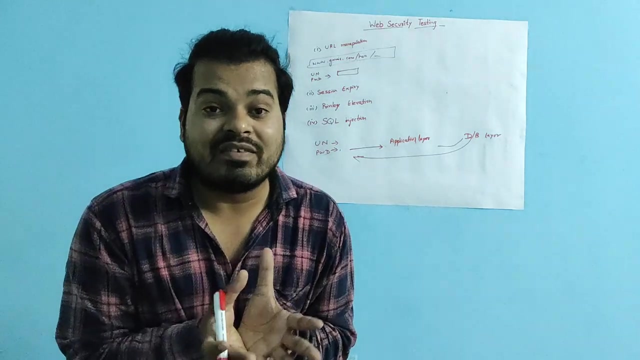 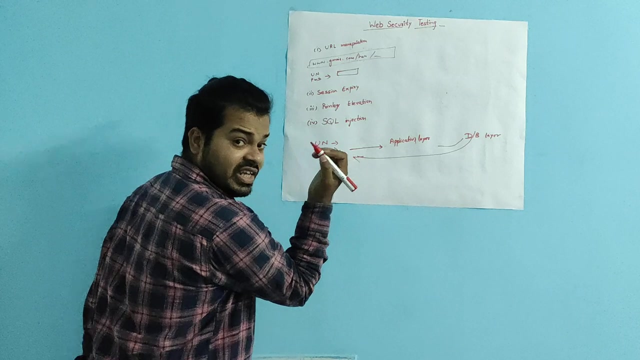 commands by which database will not understand what he is asking for and, by mistake, DB will give all the information he is having of customer information. he will give it to the hacker. This is what is called as SQL injection. Suppose his username is name, his password is 123. 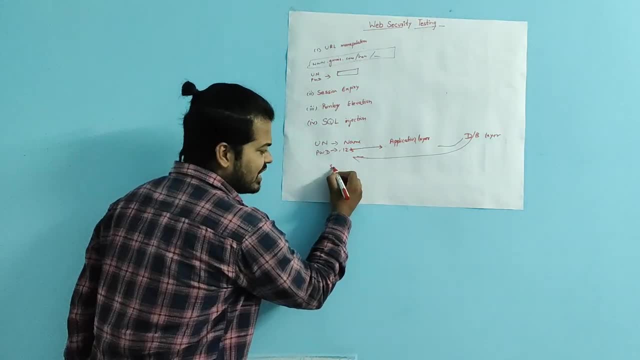 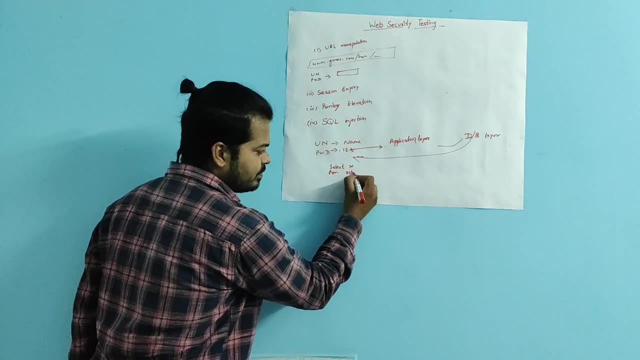 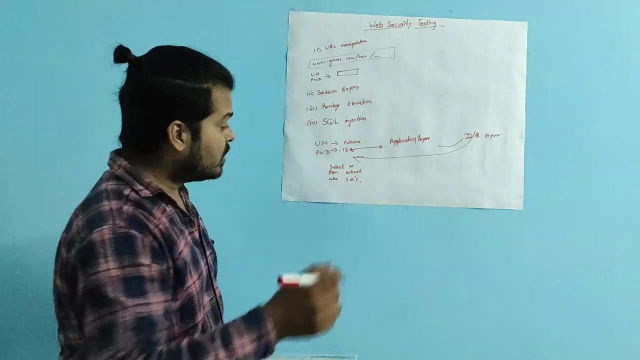 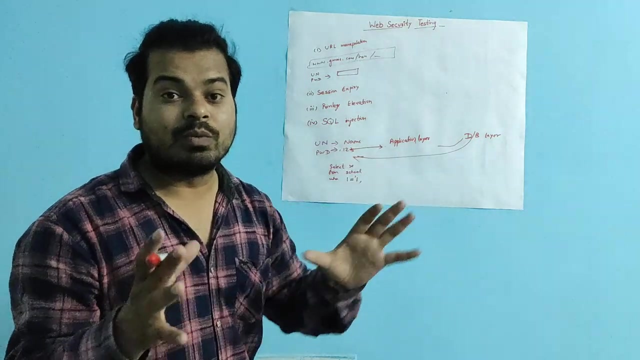 but he won't give as 123. He will give something else. Let's say SELECT star from anything: school, where 1 equals 1.. Something he will do, Something he will do additionally, which will make database to misunderstand and give all the data he is having of customer to the 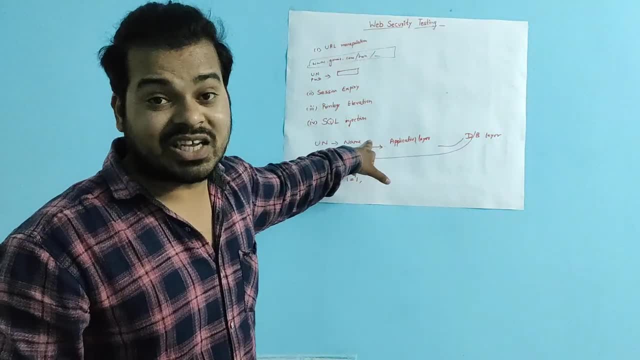 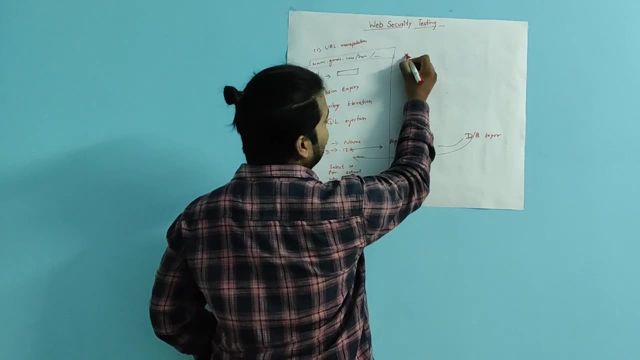 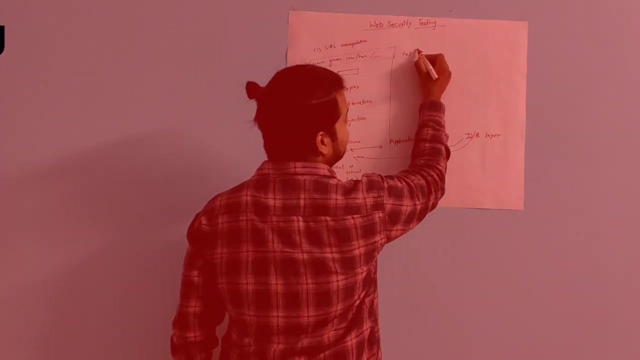 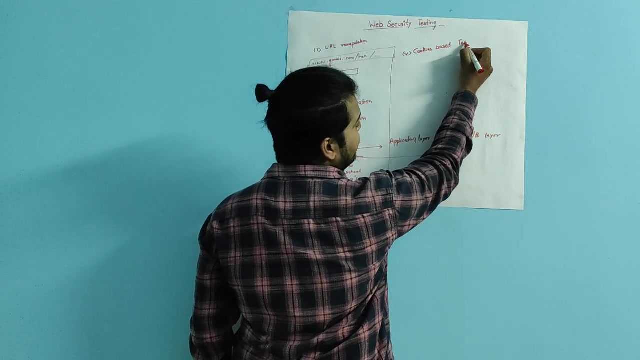 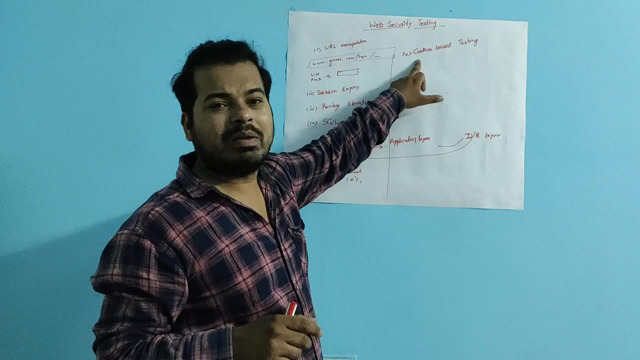 hacker. That's it. That is called as SQL injection. I hope it is clear. Let's go to the fifth type of web security testing, called as cookies based testing. Cookies based testing, Guys, cookies. What do you mean by cookies? Cookies are the piece of information sent from web server. 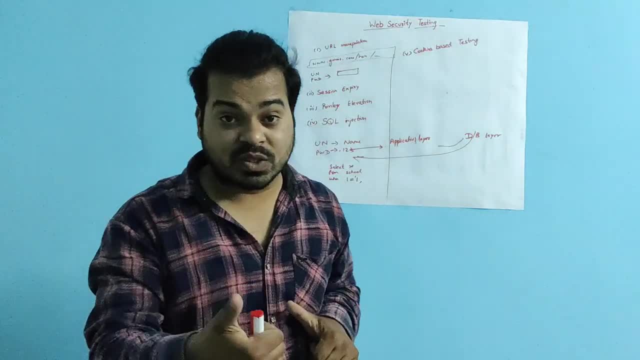 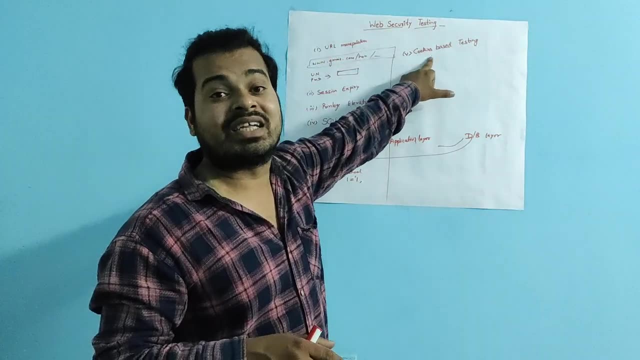 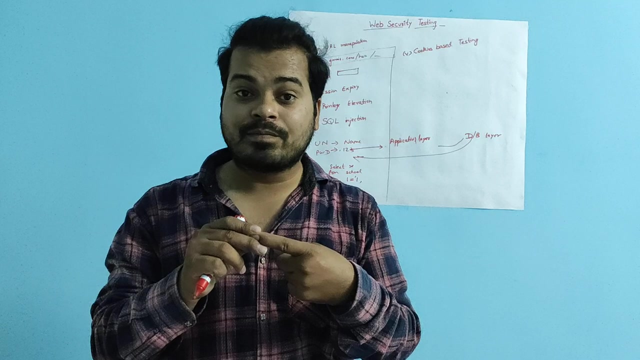 to the web browser. It can be username, It can be password, It can be my url. That is called as cookies based testing. In cookies based testing we have two types. The first one is called as session cookies and the second is called as persistent cookies. In this, 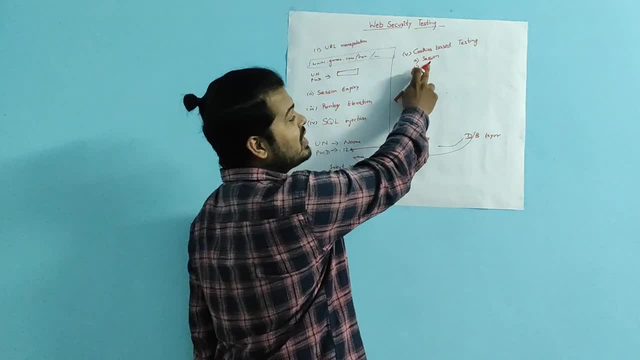 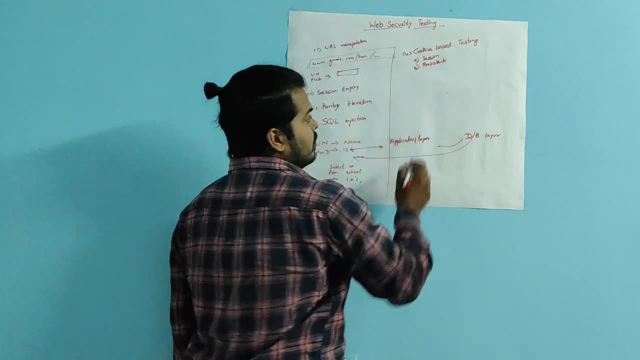 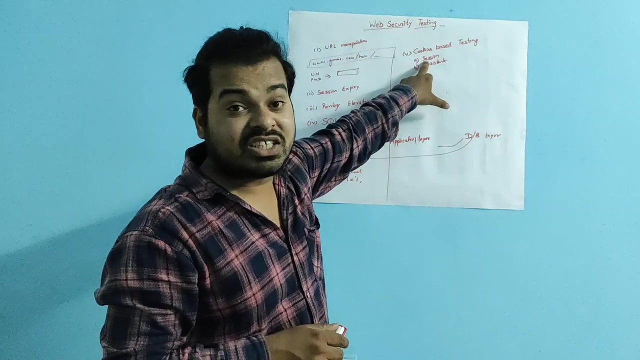 the first is called a session cookies, The second is called circuit cookies, Second one and the second part is persistent cookies. Now, what do you mean by session cookies? As the name suggests, session cookies, these are the cookies which will be stored in the 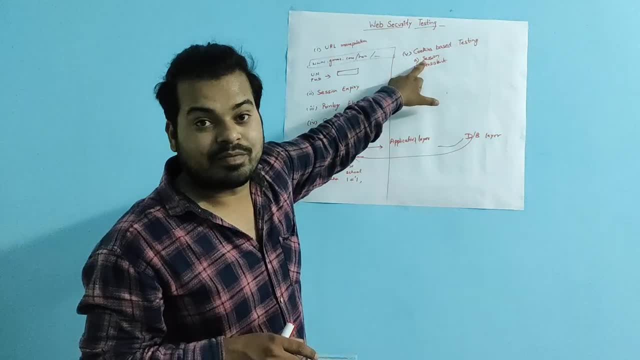 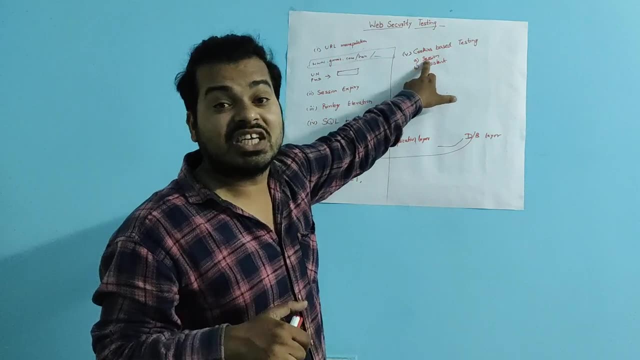 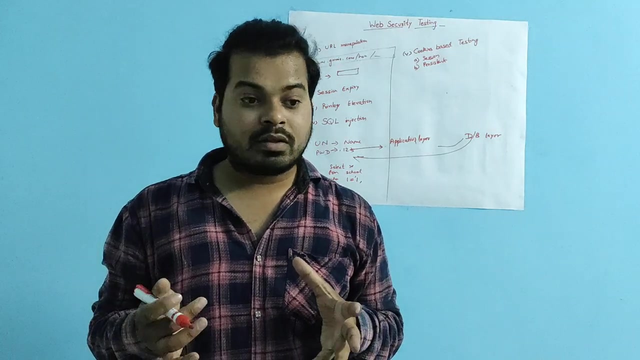 browser for a particular session. These are the cookies which will be stored in the browser itself for a particular session, In the sense when I am using any application for a particular period of time, let's say from 11.30 to 11.45,. in between that period, only the information. 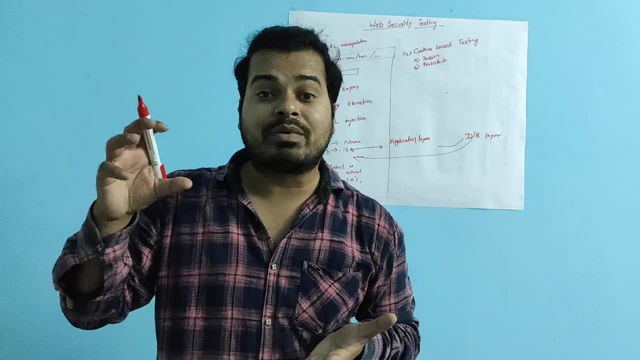 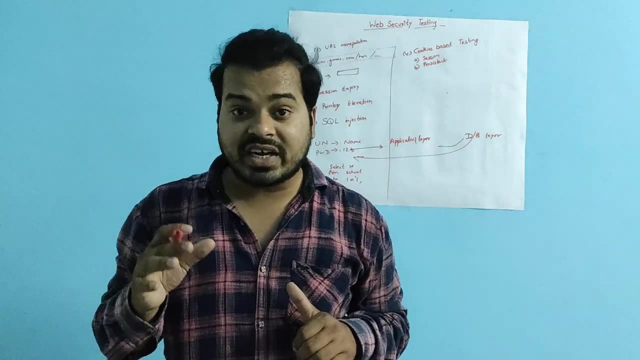 or cookies. username and password or my URL will be stored in the browser After I have closed the browser or after I have logged out from the application, or after I have shutted my application fully. the information will be stored in the browser itself. 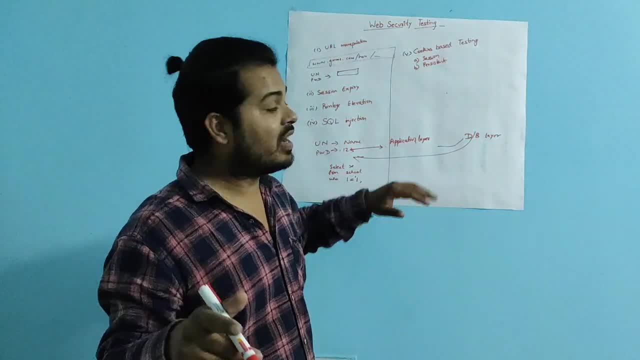 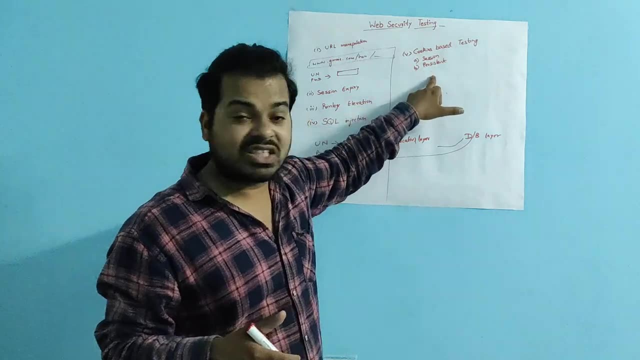 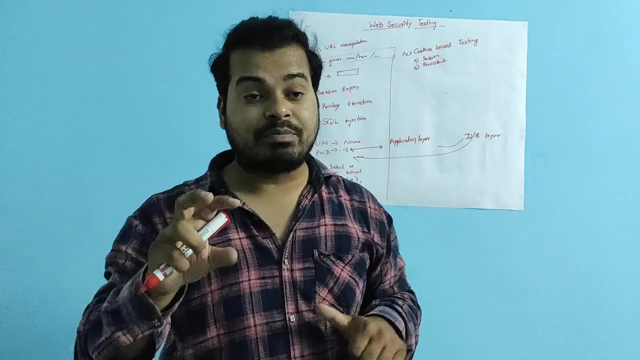 That is called as session cookies. Now the question arises: what do you mean by persistent cookies? So, persistent cookies, these are the piece of information which will be stored in the memory of your computer. These are the piece of information, persistent cookies. 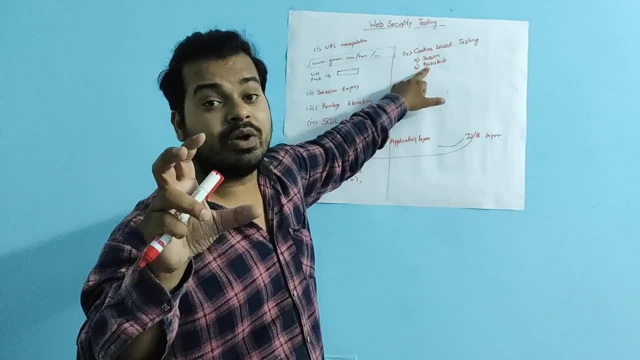 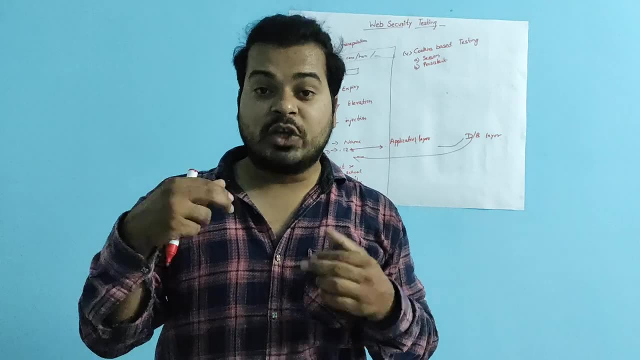 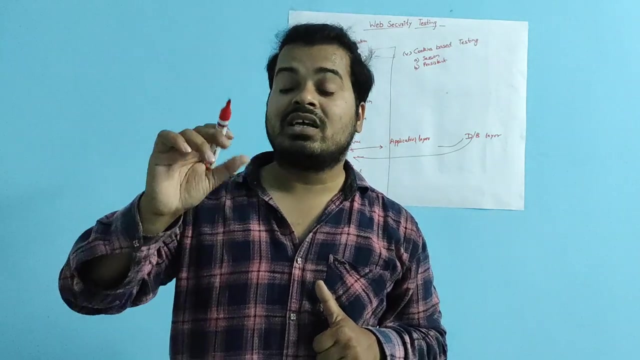 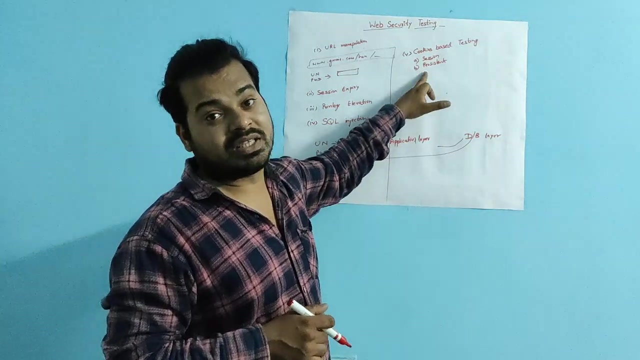 These are the piece of information which will be stored in your hard disk of your computer and it won't be deleted. User have to delete it or it gets deleted automatically after it reaches a particular expiry date. That is called as my persistent cookies. I hope it is clear, guys. Let's go. 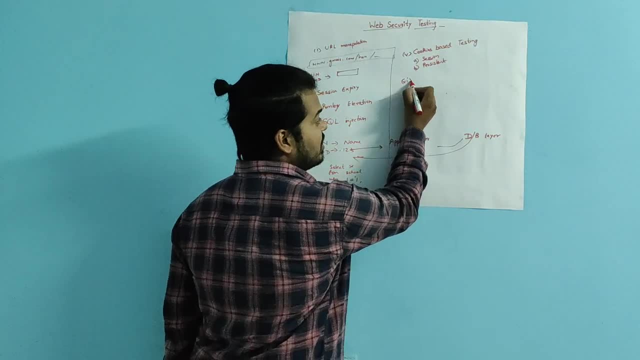 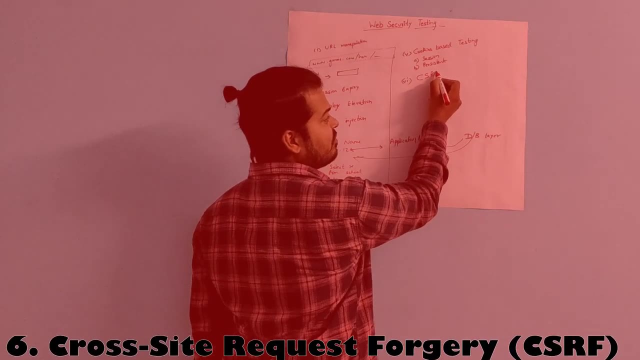 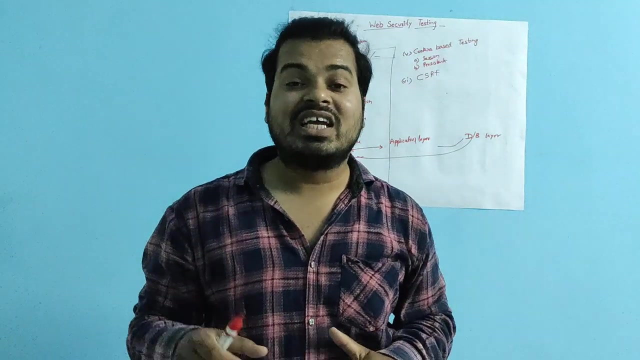 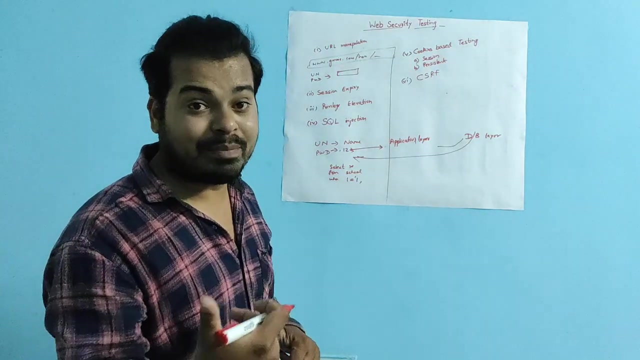 to the sixth type. Sixth type of web security testing That is called as CSRF attack. So let's go to the sixth type. First step is cross site request for forgery. We will test that URL is encrypted or not. Let's say you are using a bank application where you are trying to send the money to. 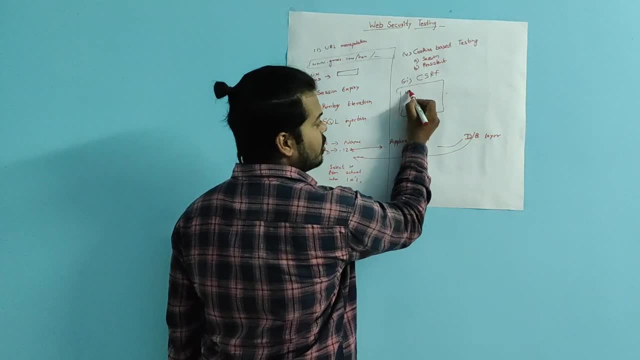 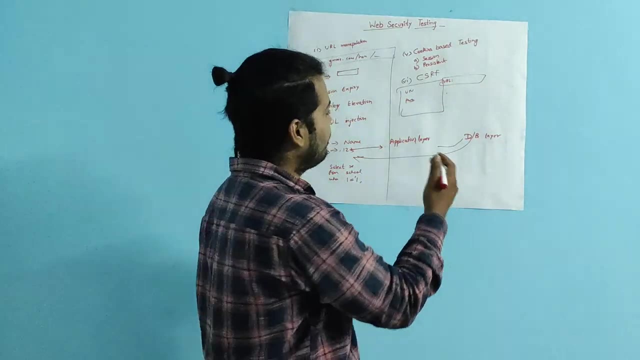 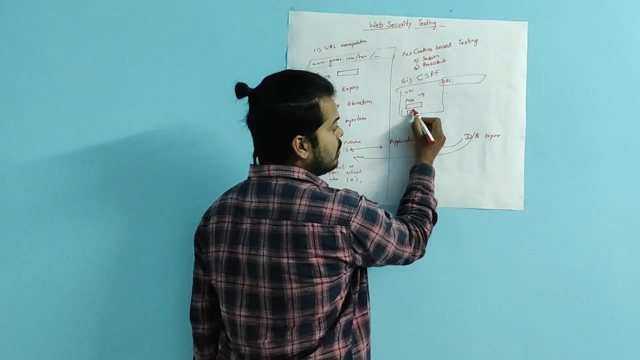 your friend. This is your bank application with your username, password and this will be your URL. Let's say You have logged in. After logged in, it'll ask how much amount you are trying to send and for the details he will ask, You will fill here Now, guys. 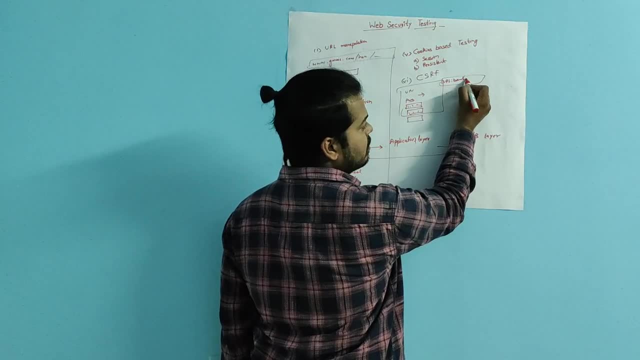 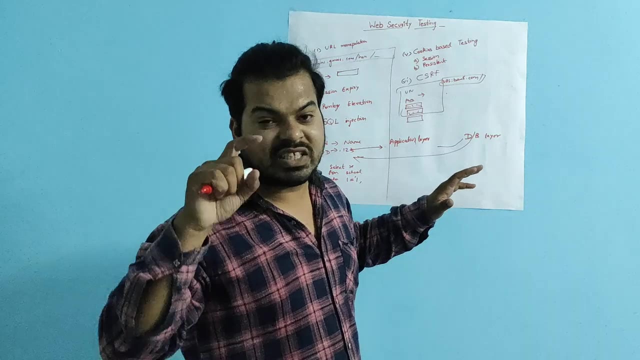 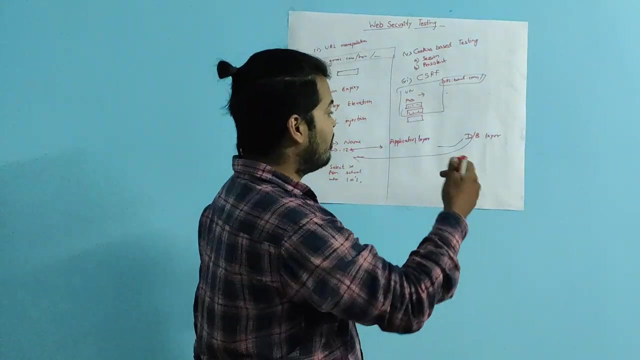 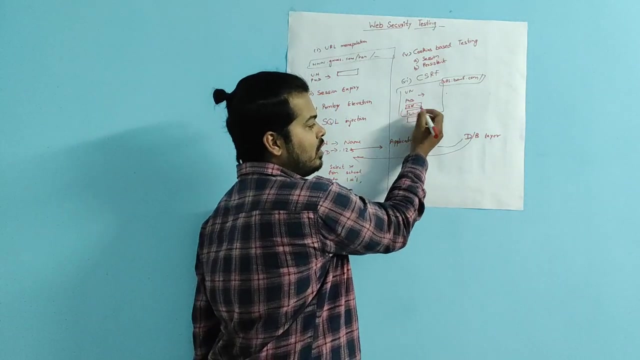 suppose you are using any bank application, Guys, you must have observed: whichever link you will try to click, your url will change according to that. So when he is trying to fill all this data, like he is sending 10 lakh rupees or whatever, or he is sending to a person. 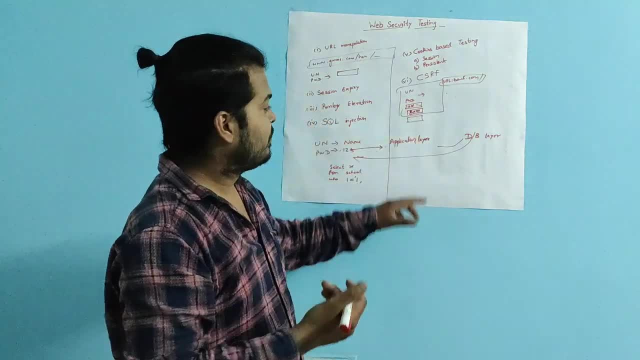 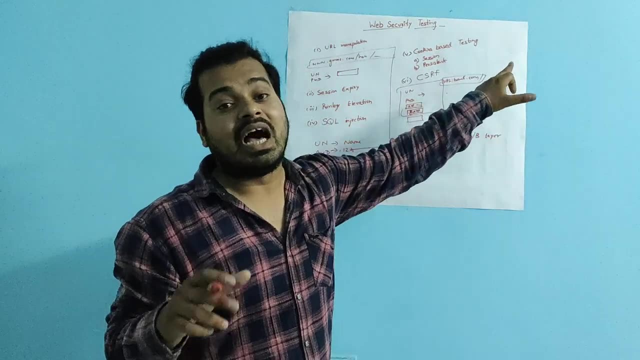 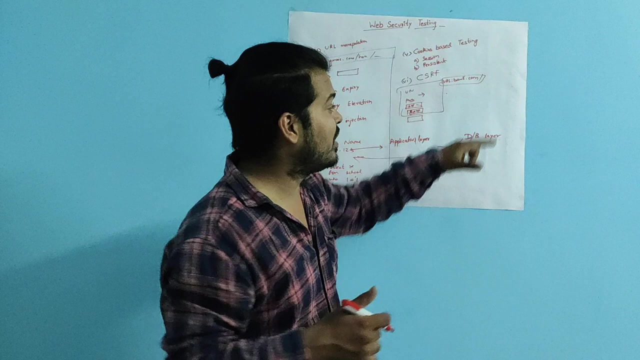 name as Ram or anyone. These are all data are my sensitive data. It should not be visible in my url. If it is present, I will say that it is a defect, Security defect- But if all this data are encrypted here- Encrypted in the sense it won't be visible, It will be. 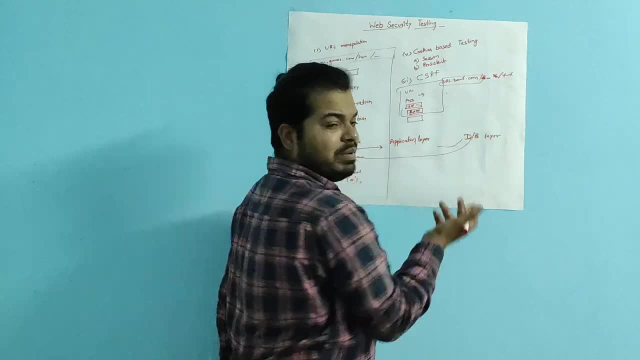 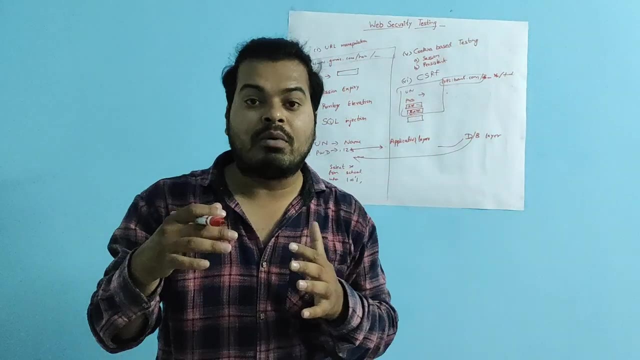 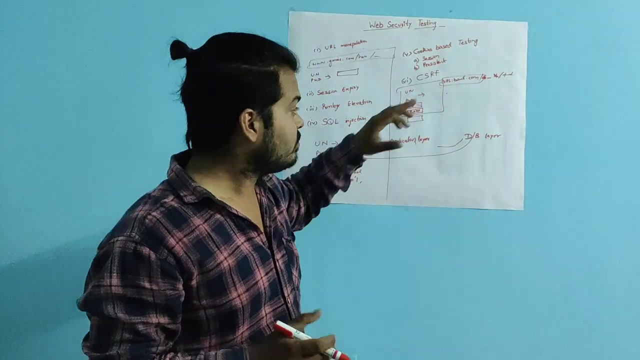 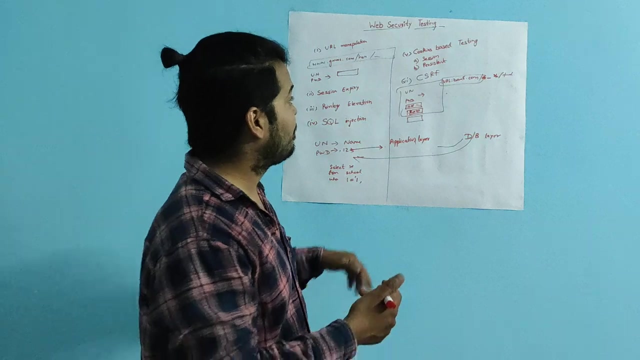 something like: It will be encrypted. It won't User. if they see the url, they won't understand that. what is the amount user is trying to send to someone? That is called, as by CSRF attack, Cross site request for forgery? I hope it is understandable. Let's go to the seventh type of web security. 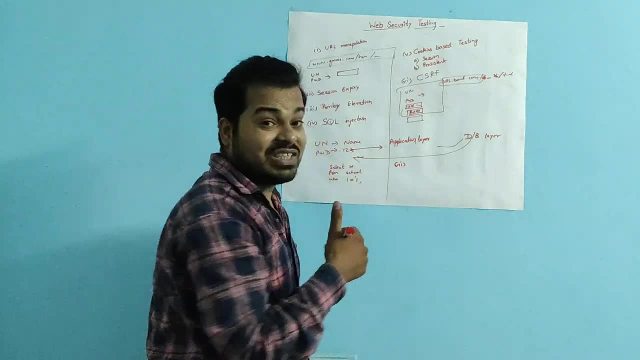 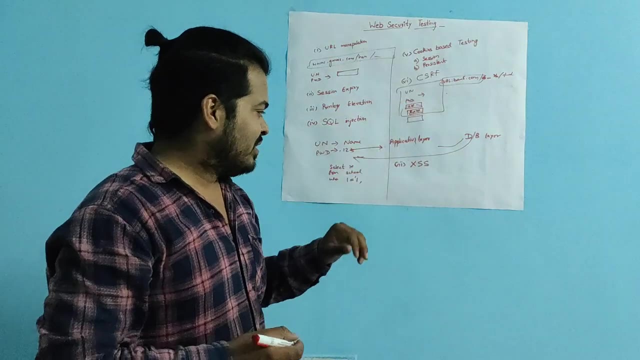 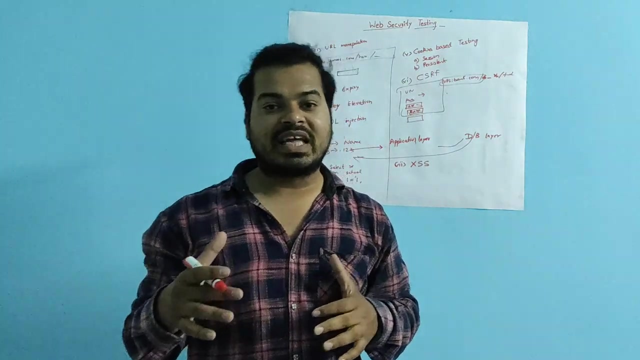 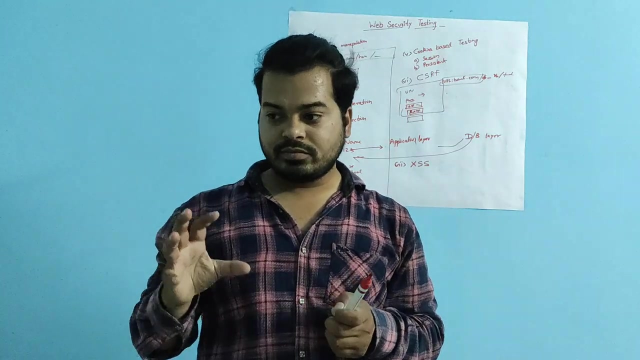 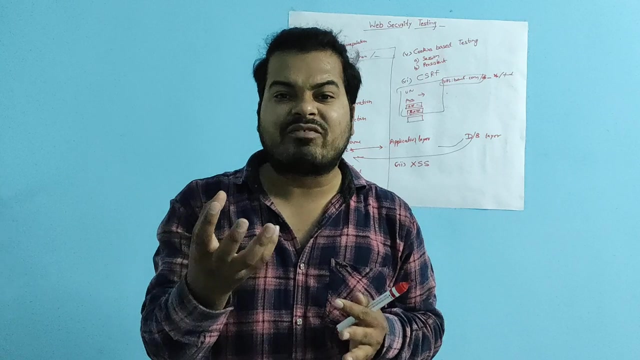 testing, Which is called as XSS attack. XSS attack- Cross site scripting. In this, Suppose you are using any application. Suppose you are using any application. When you are using it, suddenly You see something different in your application, Something which looks like a fraud Asking you to click on it. Let's say you are using 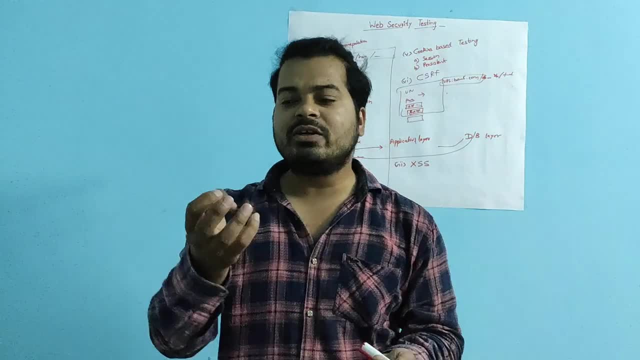 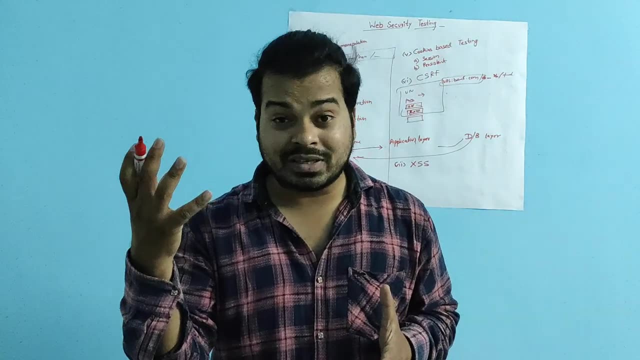 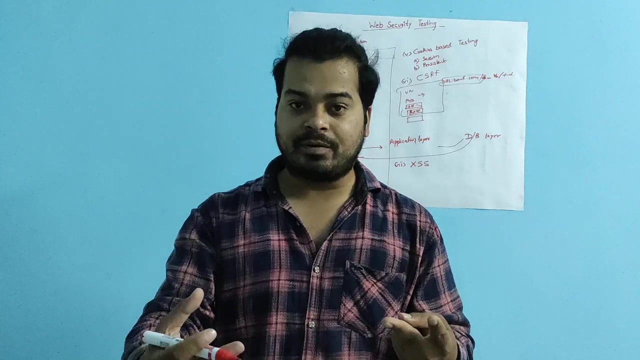 some application. You are using some bank application And suddenly you see a pop up saying that, like my images, Suppose you are using some bank application- or suddenly pop up comes as buy 2 get 5 free. Buy 2 jeans, get 5 jeans free. What user will do? User.